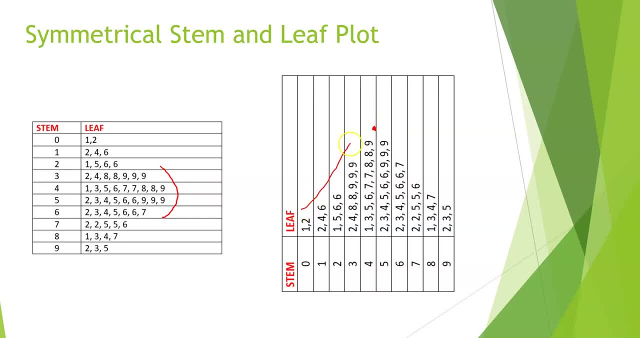 if we look at the shape of the plot, we can see that it comes to a peak here and then comes down, and it is almost perfectly symmetrical. The majority of the data values are in the centre of the plot and, as a result, the majority of the values are distributed. 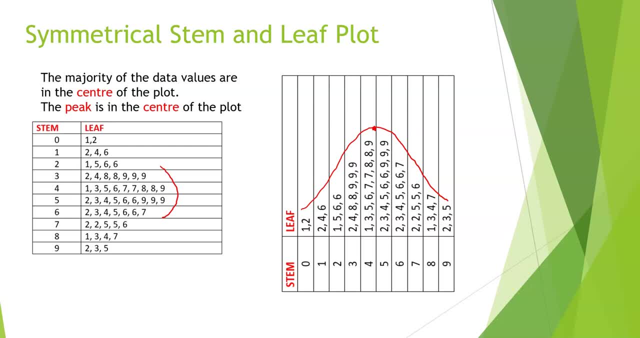 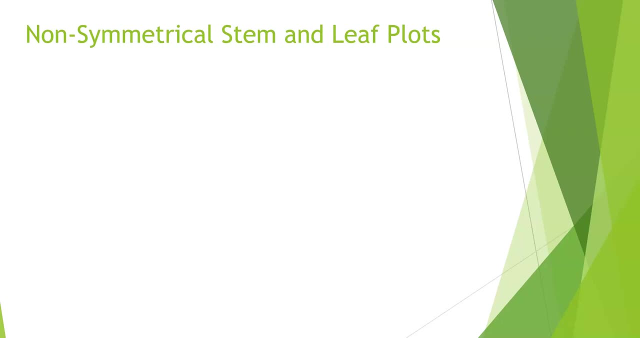 The peak of the stem and leaf plot is in the centre of the plot. This is what we call a symmetrical stem and leaf plot. Now let's look at some non-symmetrical stem and leaf plots. Let's look at this first one. 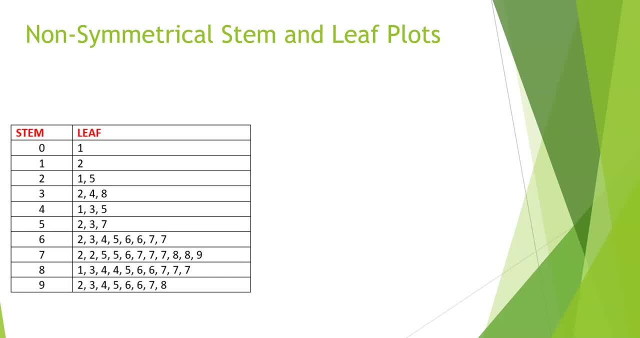 We can see now that the majority of the data is not situated in the centre of the plot. This time it is situated towards the bottom of the plot, down here. We still have some data values up the top, but not that many. So the shape of my plot looks something like this. 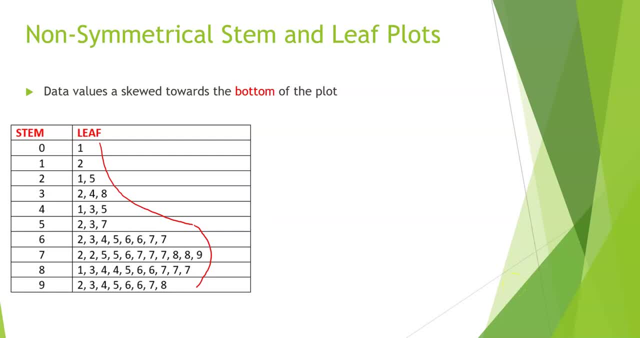 We can see that the data values are skewed towards the bottom of the plot, And when we talk about a non-symmetrical stem and leaf plot, we use this word particularly skewed. We need to talk about the plot as being skewed and which way it is skewed. 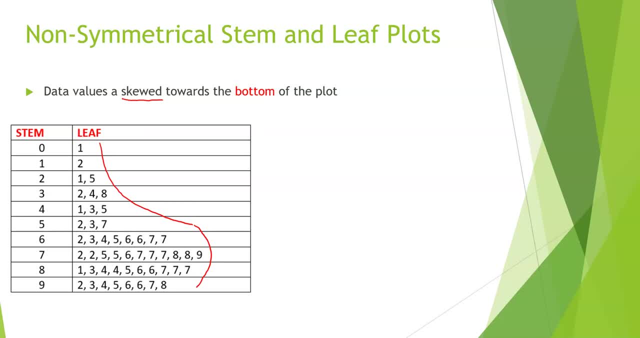 We can see that this plot here is skewed towards the bottom of the plot And we can see that the peak is situated here towards the bottom of the plot Once again, if we rotate the stem and leaf plot 90 degrees anti-clockwise. 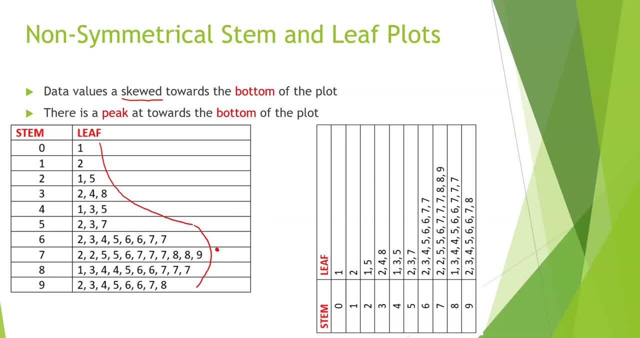 and look at it in this fashion, we can see how skewed it is. We can also see the shape. If I draw the shape over the top like this, we can see that it looks something like this: This brings us to the correct mathematical term for this type of stem and leaf plot. 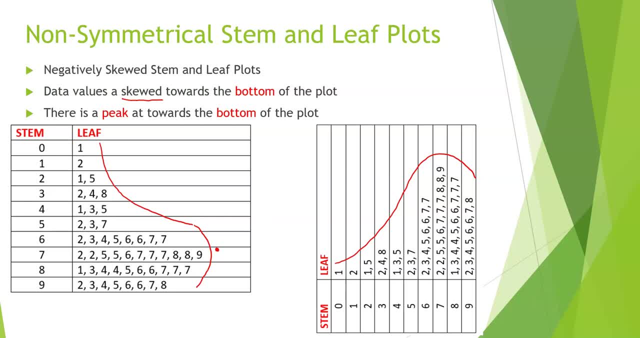 We say that it is negatively skewed. It is a negatively skewed stem and leaf plot. The reason why we say it is negatively skewed is to look at this and imagine that this line down here is like a number line, And we look particularly at the tail of the plot. 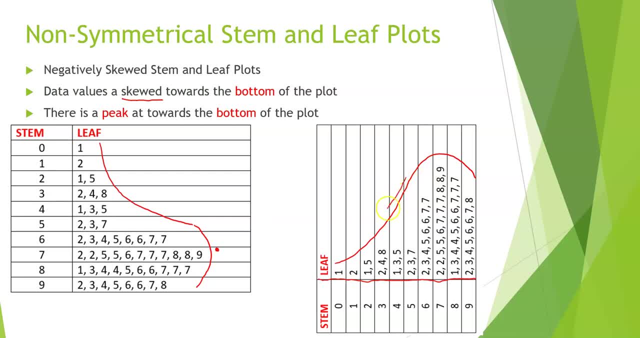 The tail of the plot is situated here And it's going in this direction, towards the left. When we can see the tail moving towards the left like this, we know that it is negatively skewed, It is pointing in a negative direction. So this stem and leaf plot is what we call negatively skewed. 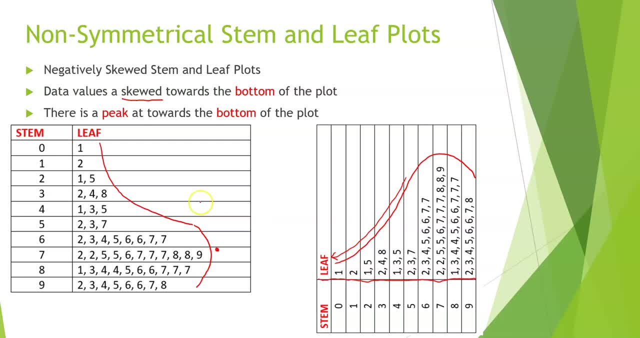 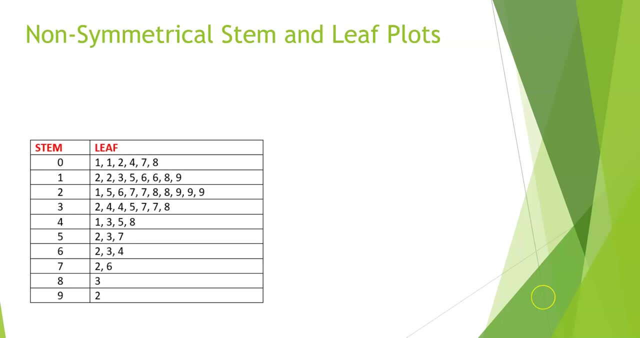 It means that the plot has the majority of the data skewed towards the bottom of the plot, And we say it's negatively skewed. Now let's look at another non-symmetrical stem and leaf plot. Again, this one is not symmetrical and we can see that the data is all situated up towards the top of the plot. 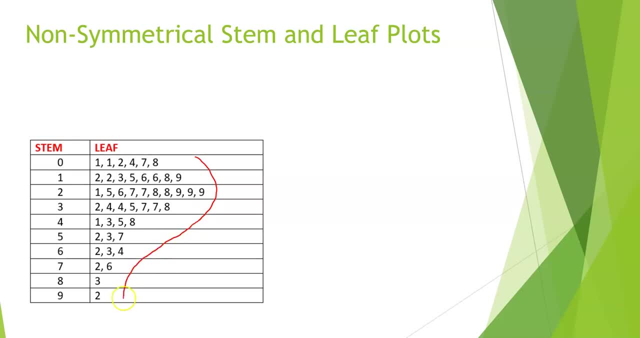 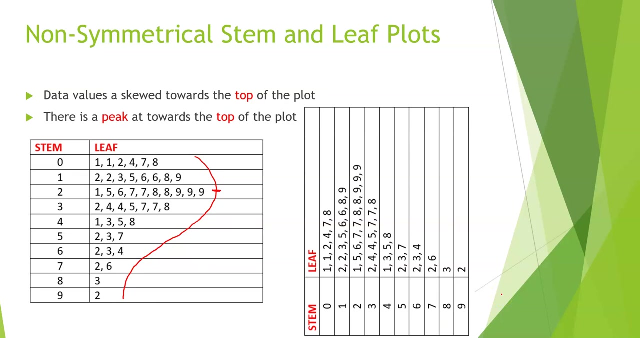 There are still some values down here, but not that many of them. The data values are skewed towards the top of the plot and we can see that the peak is towards the top of the plot as well, the peak being here Once again. if we look at this stem and leaf plot by rotating it 90 degrees anti-clockwise, we can see the shape of the plot looking like this: 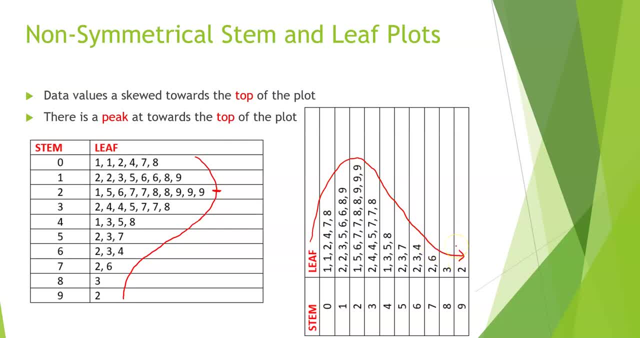 So we can see the shape of the plot looking like this Once again, look at which way the tail is pointing. The tail is on this side and pointing in a positive direction. So we say that this stem and leaf plot is positively skewed. 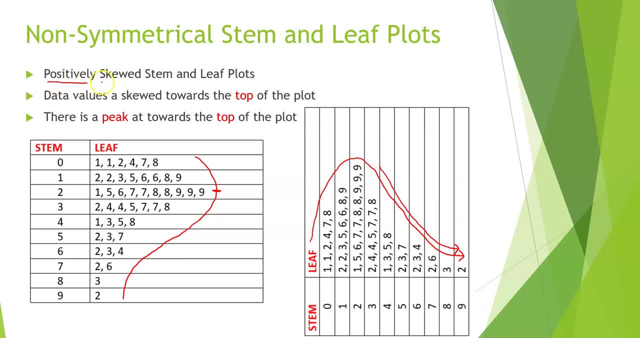 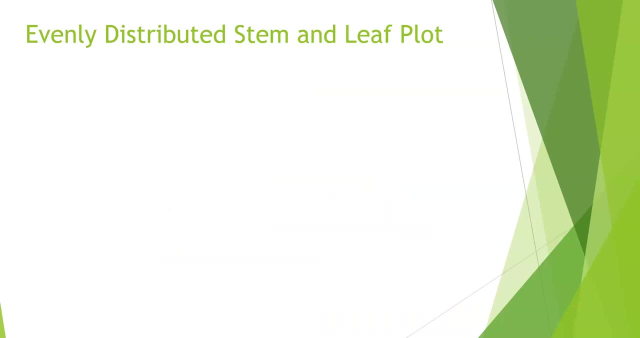 The majority of the data is all situated towards the top of the stem and leaf plot. The fourth type of stem and leaf plot that you could describe is an evenly distributed stem and leaf plot. Here is an example. You can see here that we don't really have any peak at all. 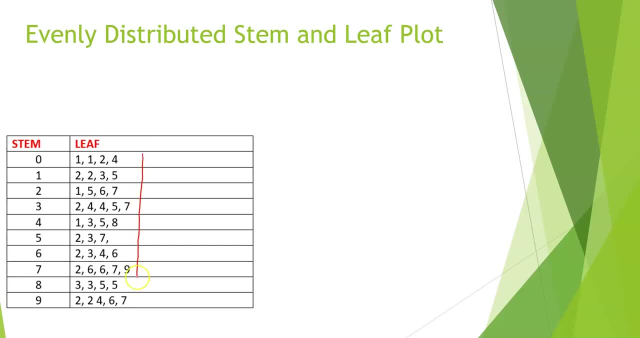 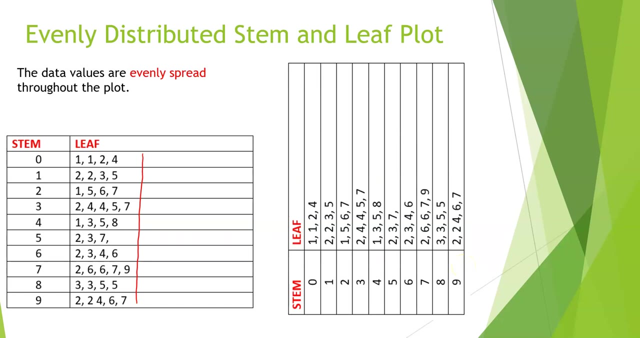 If I try and draw the shape of this, it's almost like a vertical line. The data values are evenly spread throughout the plot And if we look at the stem and leaf plot, rotated 90 degrees anti-clockwise, we can see that there certainly are no peaks. 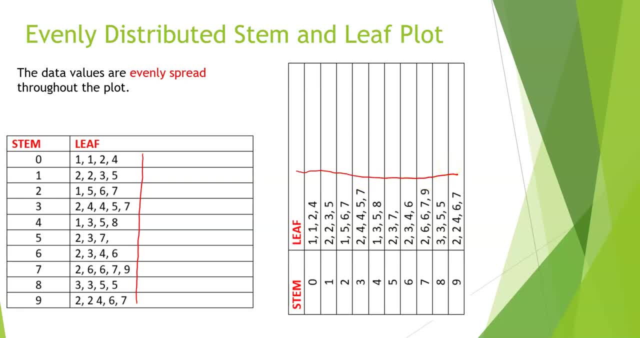 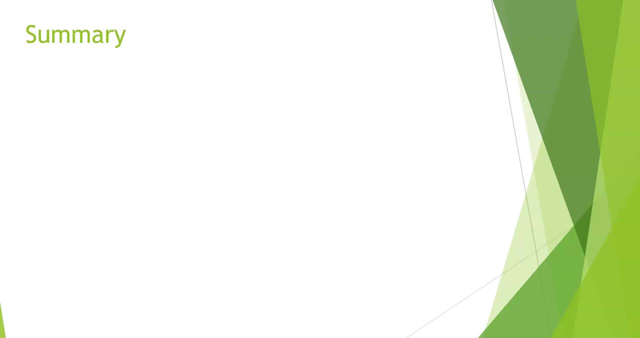 It's like a horizontal line. now There are no peaks in this distribution and therefore we say it's evenly distributed. So, in summary, when we are discussing and interpreting a stem and leaf plot, there are four different types of stem and leaf plot that you can talk about, and we describe the 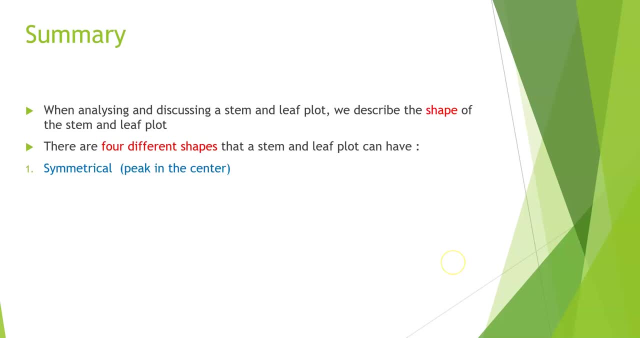 shape of the stem and leaf plot. You can have a symmetrical stem and leaf plot, which means that the peak is in the centre of the stem and leaf plot. You can have negatively skewed stem and leaf plot, which means that the peak is situated. 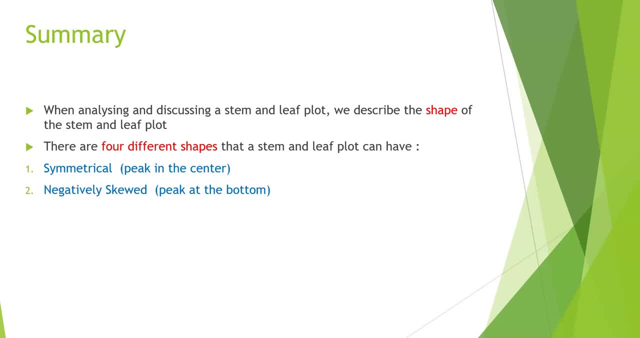 towards the bottom of the stem and leaf plot. Or you can have an evenly muscle spread stem and leaf plot which means that there is no peak there at all. When you are interpreting and discussing a stem and leaf plot, you need to talk about the shape of the plot. You need to describe whether it is symmetrical or not.